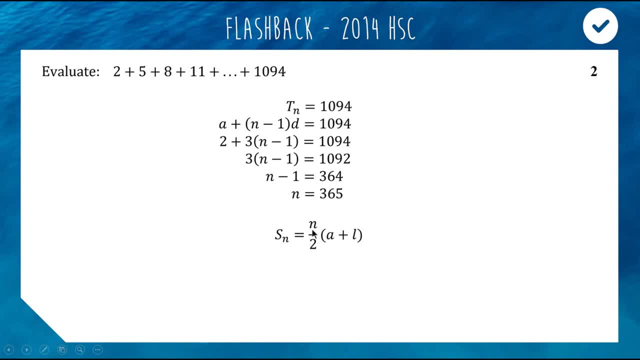 but that's all right. So we can do n over 2, n is 365.. First and last are 2 and 1094.. Put that through the old calculator and we get 22020 as the sum of this series. Okay. 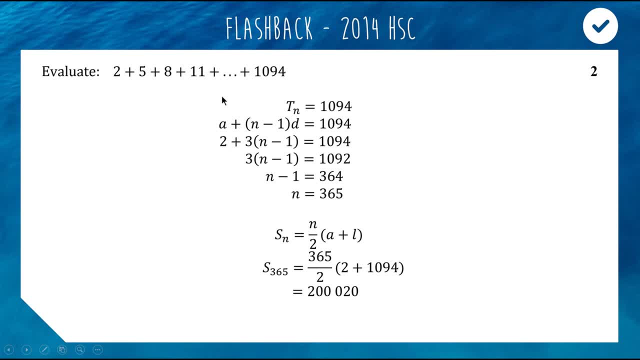 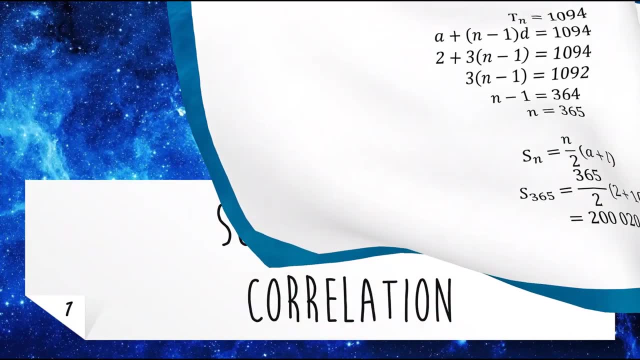 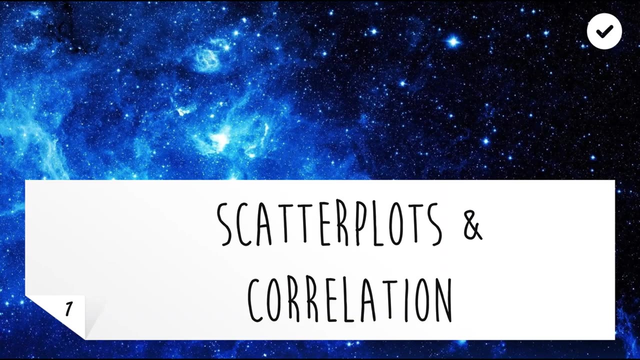 and that was much faster than putting in 365 terms into our calculator, So this is the way I recommend you approach it. All right, so today's lesson is all about scatter plots and correlation, as well as just a bit of an introduction to bivariate data. All right, so we're starting off. 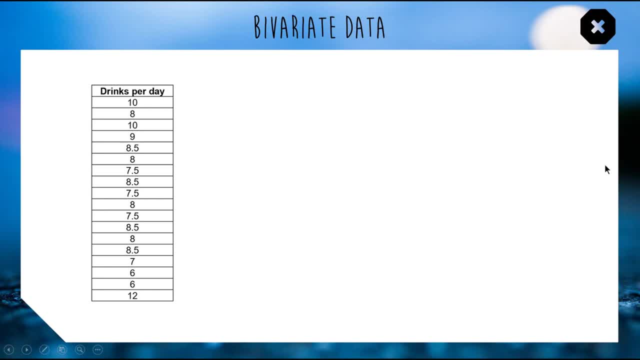 with. here is some data that I recorded over a- I believe it was an 18 day period. I recorded the number of times I had a drink of water in any specific day, All right. so on the first day I had 10 drinks of water. 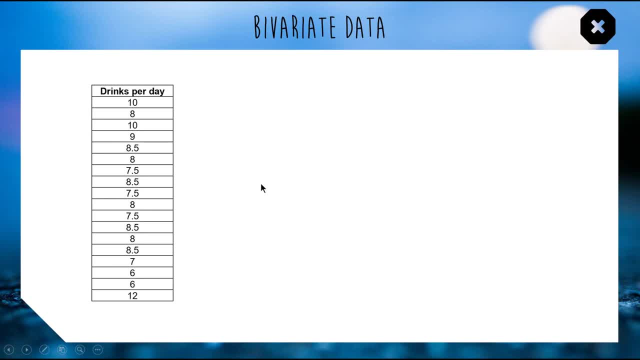 On the fifth day I had 8.5, tried to just round the nearest half glass because make it simple. Now, right there, what I've recorded is called univariate data. Okay, I've only recorded one thing, one variable, and it's not very interesting. What we look at in this topic is comparing this. 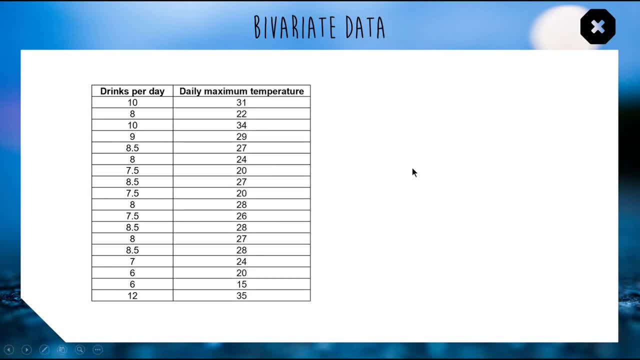 to some other variable to make bivariate data Okay. so I looked up the weather reports And on the day when I had 10 drinks of water, the max temperature in my local area was 31 degrees, So on and so forth. So when I had six drinks it was a 20 degree day. Okay, Now I was looking at this. 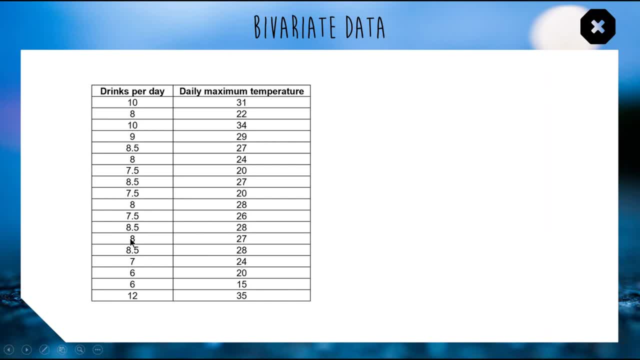 data and I was thinking: is there some sort of relationship between these two sets of data? Is this, is this data trending towards something? So I did what any normal human would do: I entered it into Excel and I created what's called a scatter plot. Okay, so I plotted all these data points as 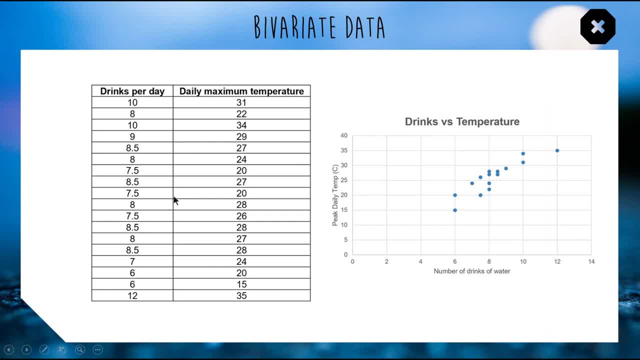 coordinates where my x axis is my number of drinks And my y axis is my peak daily temperature. Okay, And, as you can see, I wasn't crazy. there is a trend, And you can even put a trend line on your scatter plot. Okay, So this thing that I just called 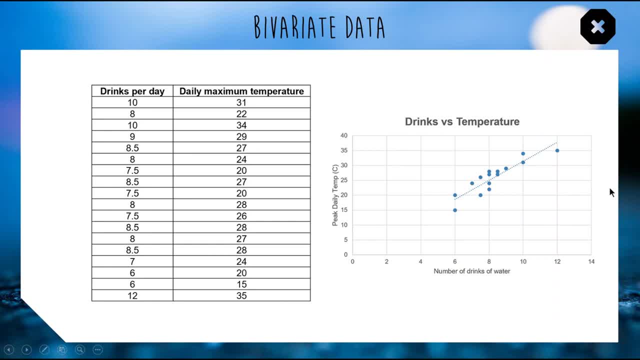 a trend line in this topic. we'll be calling it either a line of best fit or a regression line. It's a line that tries to sort of find the center of your data And so you can sort of create a model to make predictions. We'll be talking more about trend lines. 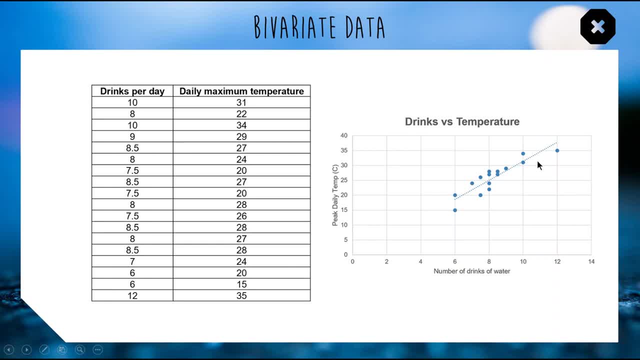 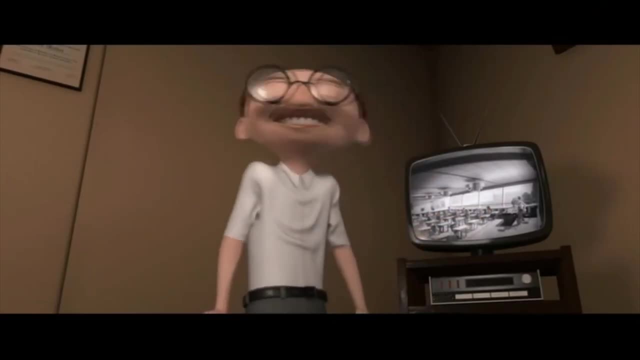 and lines of best fit in the next lesson, For this way, we're just going to focus mainly on bivariate data and scatter plots. Okay, So it's painting a pretty clear picture. these two sets of data are clearly related. Coincidence? I think not. So the only logical conclusion is that I don't really understand how, but somehow I can control the weather by how many drinks of water I have. If I drink more water, it will be hotter, So I guess you could call it a superpower, but it's not a very good one. 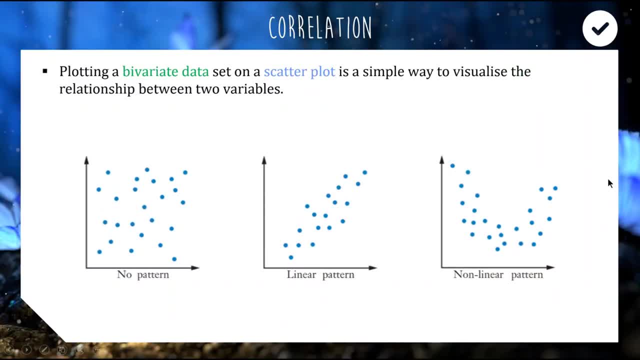 but it's interesting. So what we were seeing there is called a correlation, All right, a relationship between two variables where an increase in one increases the other, or vice versa, increasing decreases, we call it a correlation, Okay. And when you have bivariate? 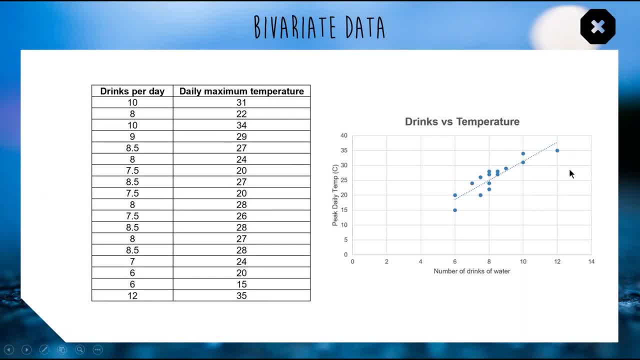 data, which is what we had before. the easiest way to try and see- it's not very clear from here, but the easiest way to see if you have a correlation is to create a scatter plot. Okay, So plot your data as coordinates. look for a trend. 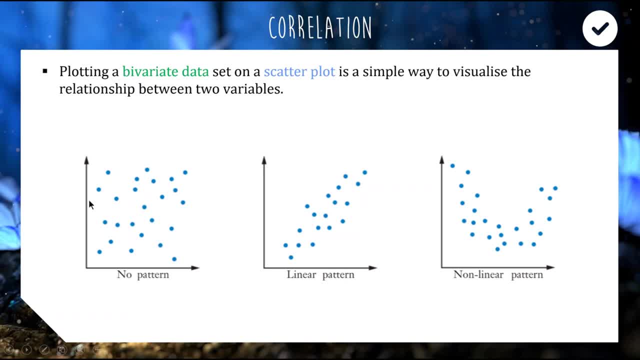 We can have scatter plots that have no linear patterns, so nothing really happening. We can have some sort of trend, like I had, a linear pattern, or we can have a non-linear pattern, which means not straight line, basically, Yeah, as I said, a correlation just means that there is a linear relationship between. 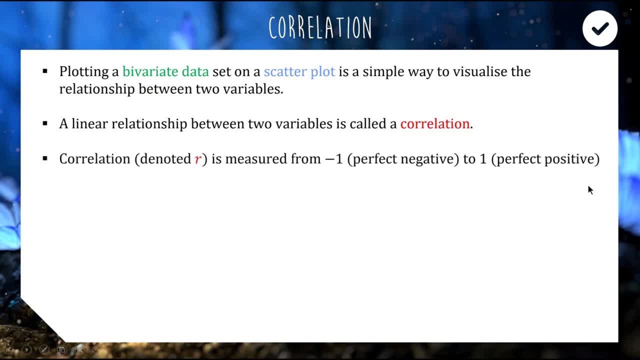 the two variables. This is just the key points of the lesson. We have a symbol- I guess you could call it- to denote correlation, because correlation is a description, but it's also actually a statistic. Okay, You can calculate how correlated a data set is. 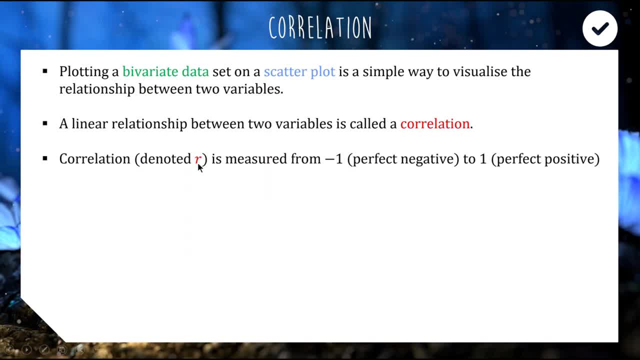 All right. And that statistic is represented by a lowercase r, and that value can range from negative one to positive one. So here's what I mean: If you had a data set that had no correlation, so there was no clear sort of pattern or trend. 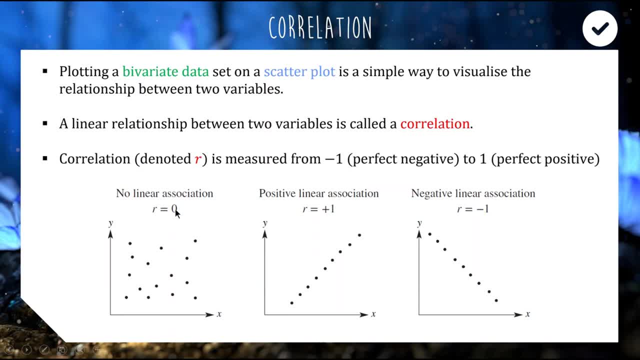 you would have a correlation value of r equals zero. Okay, If you had a data set that was showing a perfectly straight line. so you've got a perfect correlation. increasing one always increases the other. you would have a correlation value of plus one. Okay, So these are values that you can get with a calculator, which we will do later on. 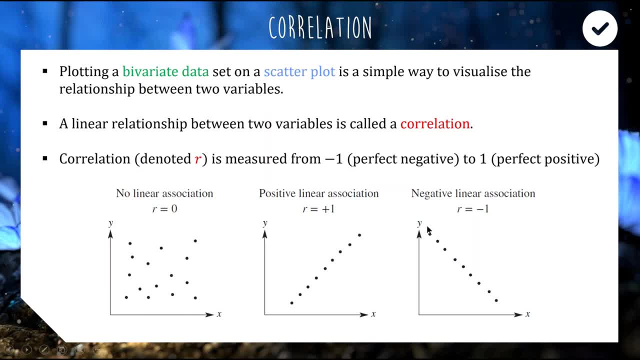 but for now we're just going to sort of estimate. And of course, if you had a perfectly straight line, but increasing one variable decreases the other, this is a negative linear association, And if it's a perfectly straight line you'll get an r value of negative one. Okay, So there's our spectrum. We range from negative one. 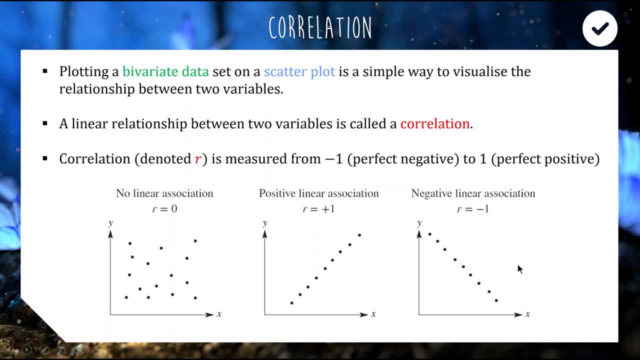 through to zero to positive one, And these are our extremes. Okay, We can be in between here, If we're. if we have some, some correlation, but not necessarily a perfect correlation. it could look like this: So this could be a scatterplot where we have about 0.3.. So it is. 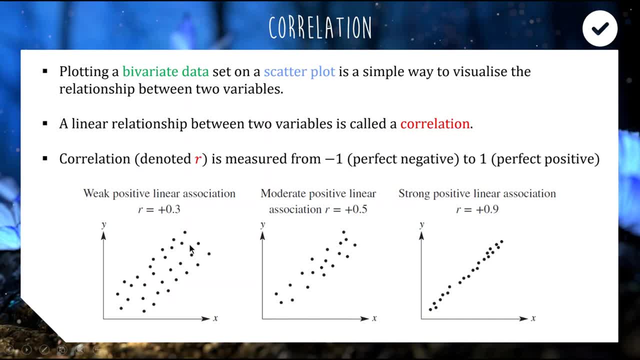 positive. It's just weak because they're very spread out, not a very straight line, And as you get closer and closer to one, your scatterplot becomes more and more consistent and you eventually will end up with very consistent, straight data. Okay, So that's correlation. We can either estimate it based off a scatterplot. 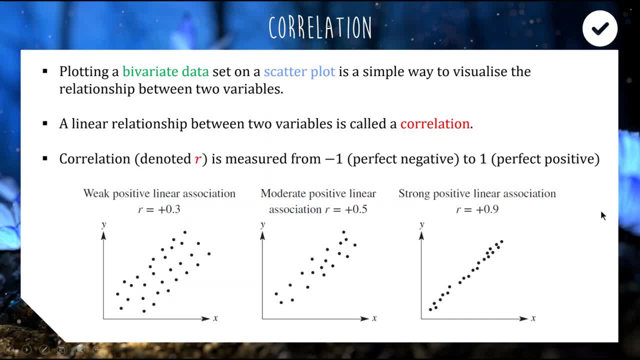 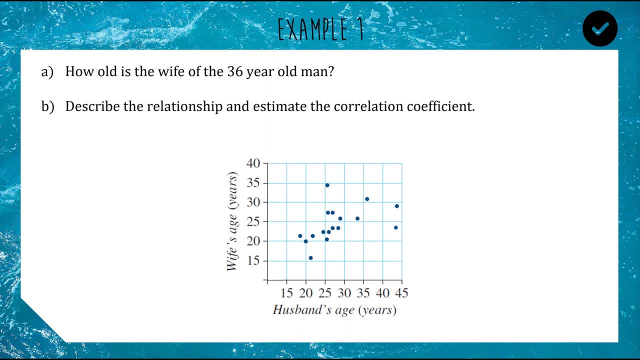 or we can calculate it with a calculator, which we'll do later on. So let's have a go at a quick example. We've got a scatterplot down here. We have on the X axis the age of the husband and on the Y axis 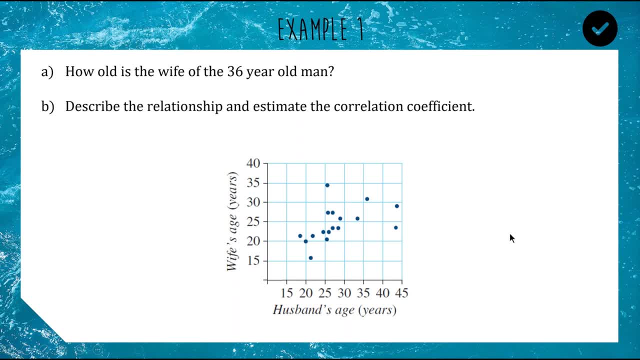 the age of the wife. Okay, So we can see a bit of a trend here. Typically, older men have older wives. We do have a couple of- uh, what you could call outliers. I guess you've got your got your Cougar value up. 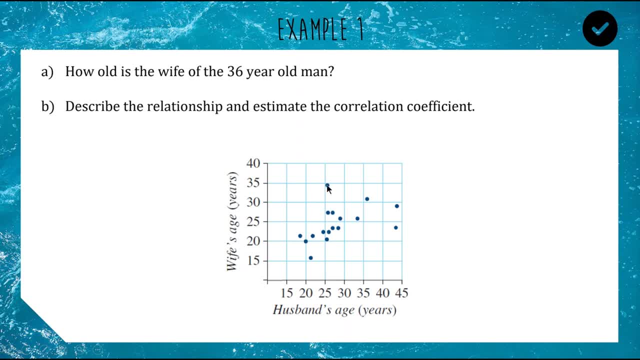 here This is the older woman with the younger husband. That's the statistical term, the Cougar value, And down here we have what's called the cradle snatcher value. We have an older man with a younger wife. but you know, love is love and all that. So, reading off this scatterplot, 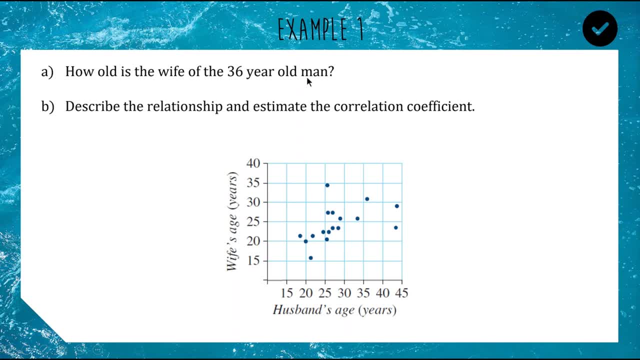 how old is the wife of the 36 year old man? Let's have a look. The 36 year old man is- this point right here- 36 on the X axis, And his wife's age is just above 30. So we'll say 31.. Okay, Describe the. 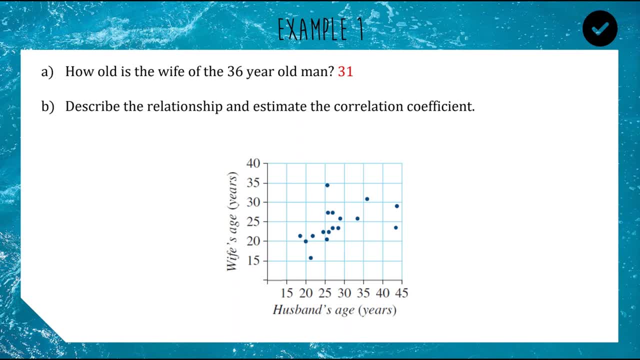 relationship and estimate the correlation coefficient. Well, like I said, there is a somewhat clear positive trend. It's not perfect though, because of these outliers and this scatterplot is not very consistent. Uh, if I was estimating it, I'd say it'd be around 0.6, but it could be closer to 0.5.. It's hard to say. 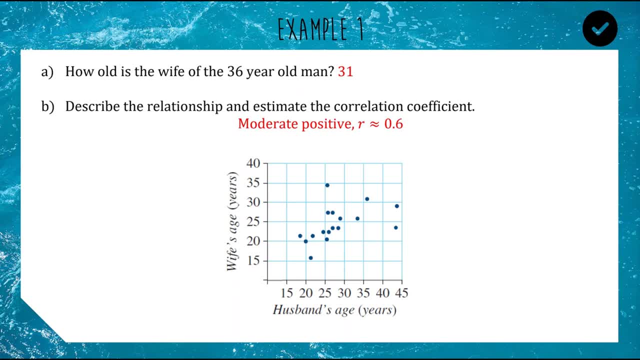 if you want to check perfectly, you can um put them into a calculator and see, but it's just an estimate. I know it's going to be around 0.5 or 0.6.. Okay, And so we would say that is a moderate. 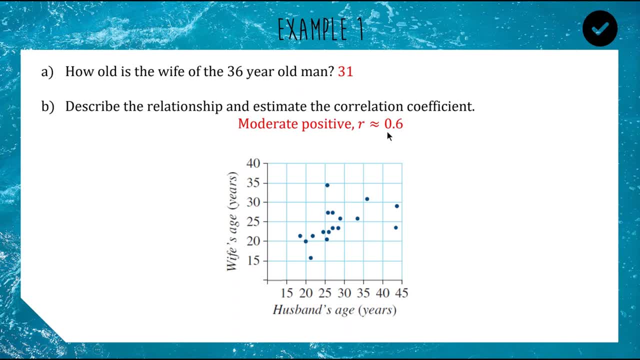 positive relationship. If that was closer to, say, 0.3, we'd call it a weak positive, And if it was closer to 0.8 or 0.9, we would call it a strong positive relationship. Okay, And again I know it's positive, not negative, because both values are increasing. 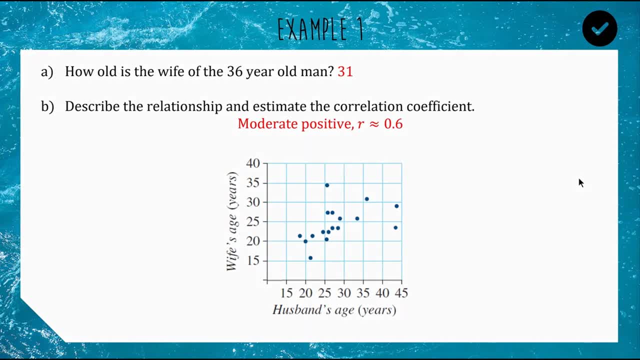 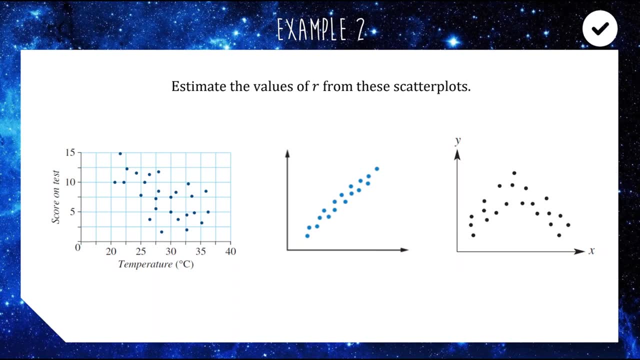 Okay, Sweet. Now for the next one. this is your uh, bread and butter HSC multiple choice question. They'll give you a scatterplot and say: pick the value of R. You don't have multiple choice. I want you to just think about pause the video and think how you would rate these uh, these scatterplots. 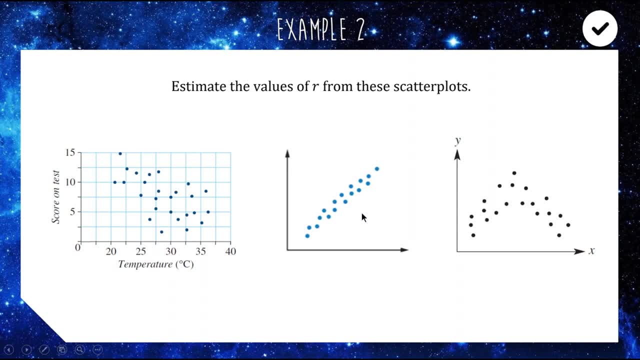 in terms of correlation from negative one to one. And I want you to think hard about this one because it's a bit weird, because it's kind of non-linear, All right. So pause and have a guess, All right. For the first one I would say it is. 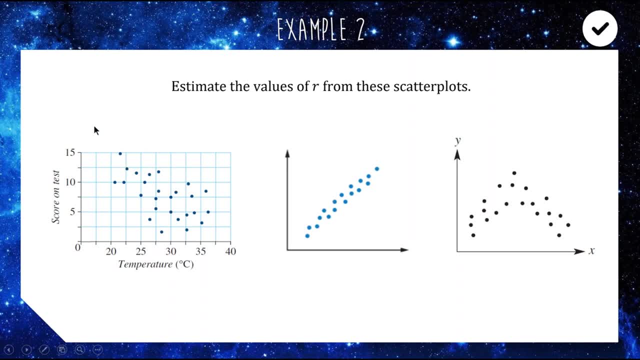 is a negative correlation and it's fairly weak. I'd be putting it probably around negative 0.3.. Okay, So if you said anything around negative 0.2 to negative 0.4, you probably get a pass mark for that. For the second one, it is positive and it's pretty consistent. It's almost. 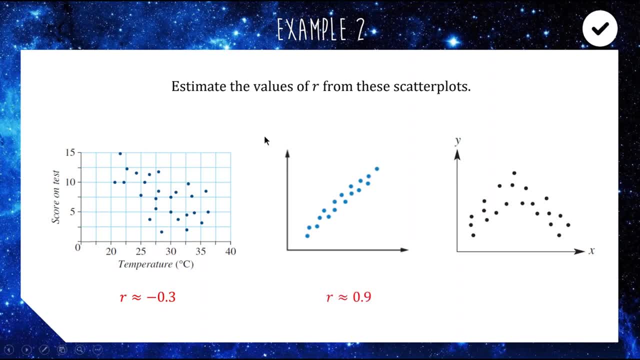 making sense. So if you said anything around negative 0.2 to negative 0.4, you probably get a straight line. I'd be putting that close to positive 0.9.. Okay, And now for Y, trying to look. 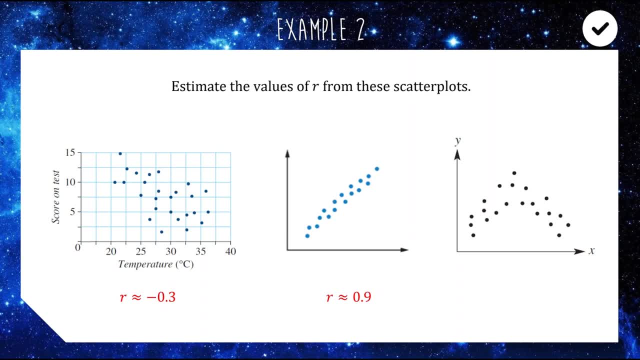 at, uh, non-linear scatterplots with correlation gets a bit weird because correlation is technically a linear calculation. So what I mean by that is if you look at this left half, you've got like maybe a 0.7, but then on this right half you've got a negative 0.7.. And so the whole thing averages. 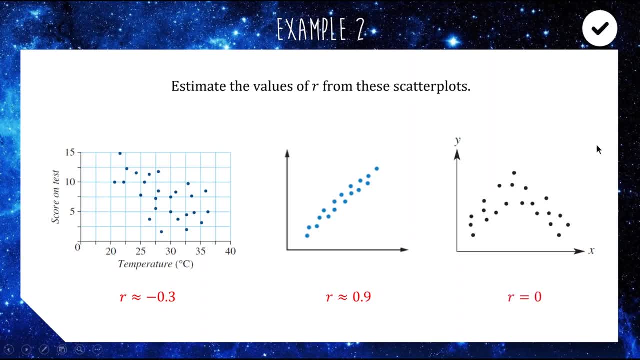 out to a zero. Okay, So if you have a non-linear scatterplot where you've got half increasing and half decreasing, the overall average correlation is going to be close to zero. Okay, So typically we'll only ask this for linear examples. All right, Now the last bit to today's lesson is: 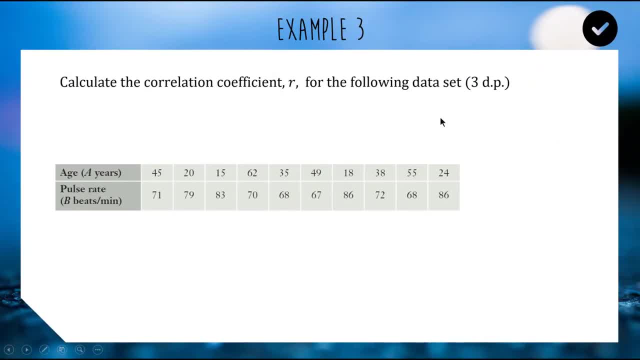 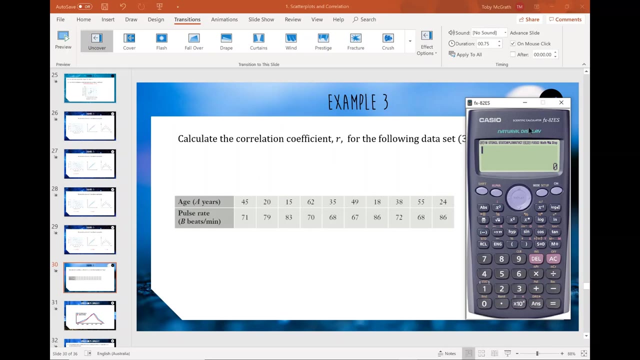 I'm going to show you how to use your calculator on stats mode to actually calculate the value of the correlation coefficient R. All right, So I'm just going to switch modes and get my calculator up, So just bear with me. All right, Here is my Casio emulator. Again, mine is a little. 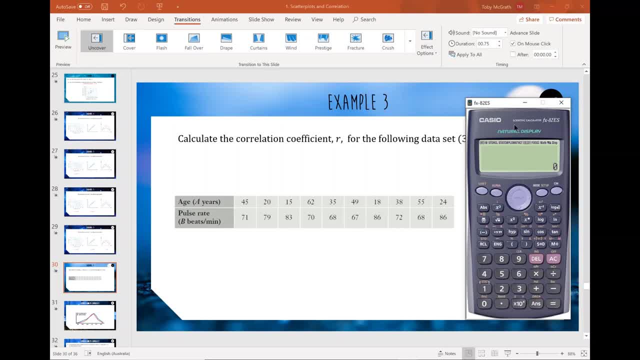 bit older than yours but it still does most of the same stuff, which is, some of the buttons might be in different spots, but you can figure it out, Okay. So first thing we need to do is enter our bivariate data. So the way we do that is we go into mode and we go stats mode again In the last. 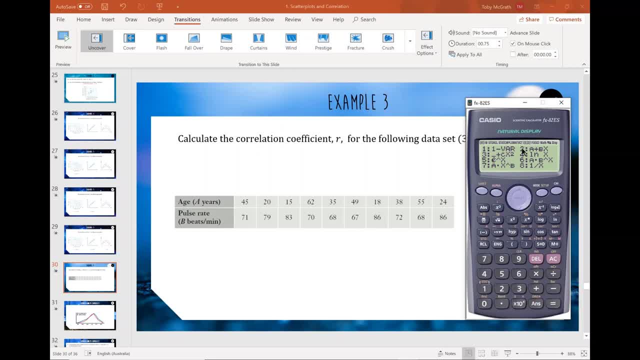 topic. we did one for single variable data. Now we are doing option two for um bivariate data. This A plus BX will make much more sense next lesson, but for now just trust me that two is bivariate data And here it is X and Y coordinates, If you still have frequency turned. 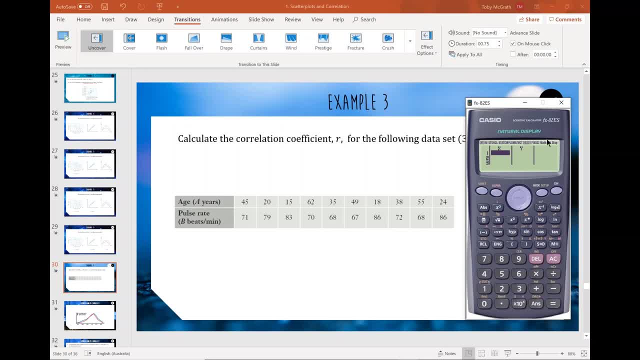 on from last time, you may have a frequency column, but for today we won't need that. All right, So we can go through. you can enter in all your X's and then all your Y's, just make sure that they all match up in pairs. So the 45 is with the 71, and so on and so forth. So I'll. 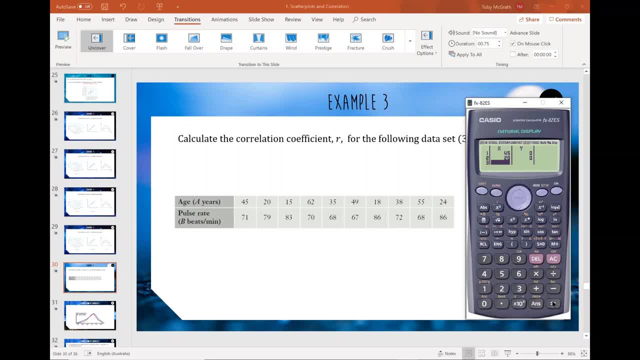 go with up 20,, 15,, fly a long at home. This is entertaining viewing, isn't it? Alright, now I've got my 10 data points for X, so I'll go to the top and I'll enter in all the Y values as well, making sure they all match up. so we've got 71.. 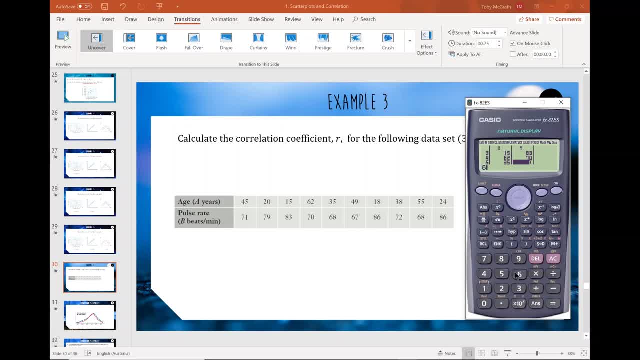 Chances I make a mistake here and don't notice it are pretty high, so let me know in the comments if I make a blunder. that's right. 67, 86, 72, 68, so close, I think, and 86, alrighty. 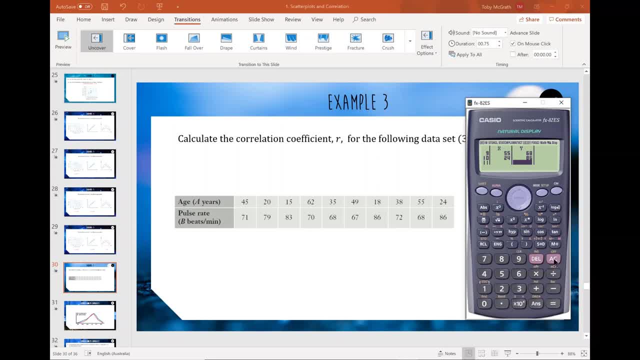 Now that our data is stored in. we just press AC to go back to the home screen, But, as always, the data is stored in there. Now we're looking for a statistic. R is a statistic, so we're going to shift one to. 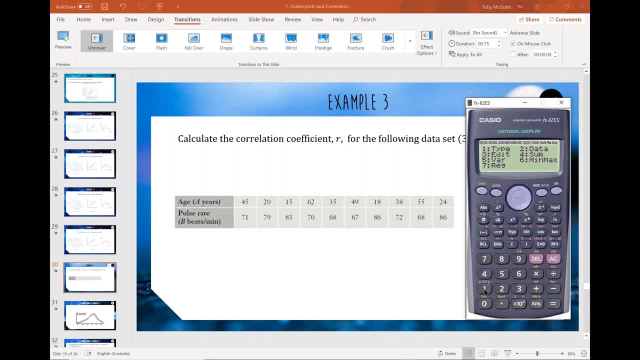 go for the stats menu Now, because we're in two variable mode. we do have more options. Yours might be in different spots, but either way, we're both looking for the same thing, which is REG, which represents regression. Again, that word might make more sense next lesson, but for now, just trust me, we're looking. 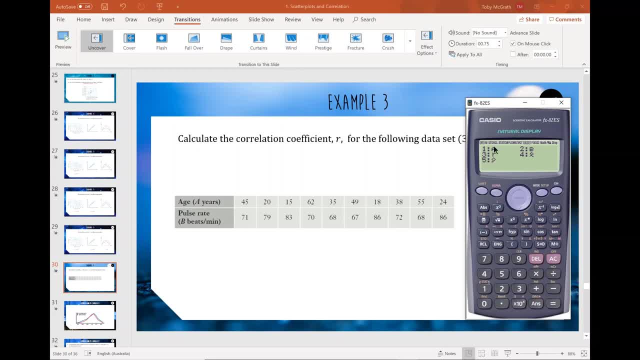 for REG A and B We'll be using NEXTTIME. you can get the X mean and you can get the Y mean, but for today we want the correlation coefficient R, so I'll press 3, tell me what it equals. it is. 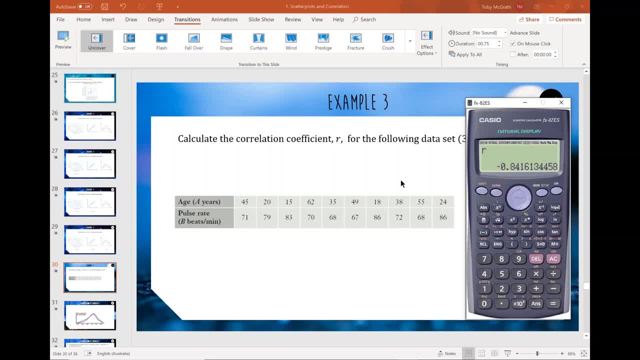 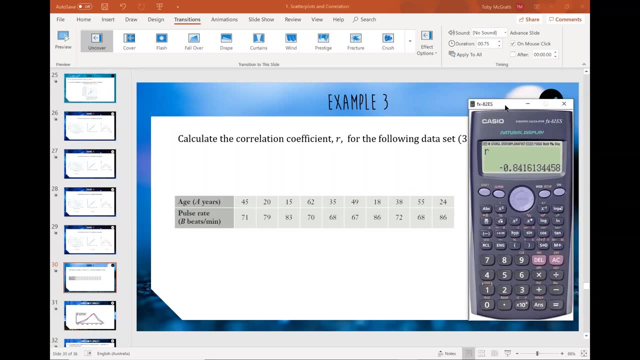 negative 0.84. blahdy, blahdy blah. So this data set has a pretty strong negative correlation. okay, So to the question one: in three decimal places, that'd be negative 0.842.. Okay, so that's how you do it, piece of cake, as long as you can remember how to get through. 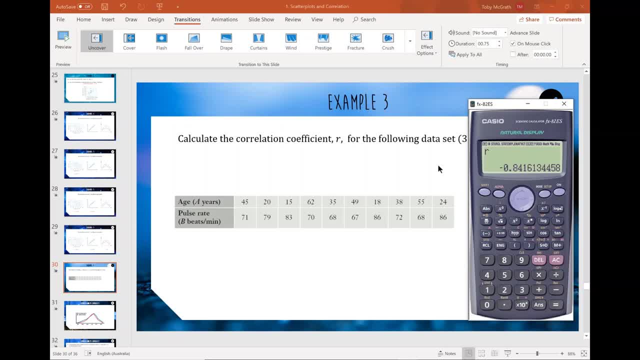 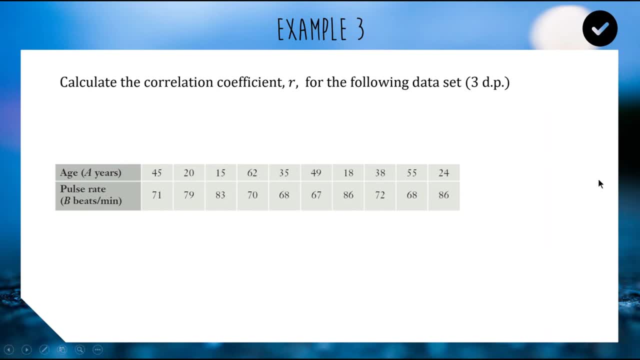 all the options in the menu. Sometimes you're going to have to fumble around, but you will find it eventually. okay, Cool, All right, and to finish off, today, we can't ever talk about correlation without getting causation involved, so I want to talk about the difference between those two. 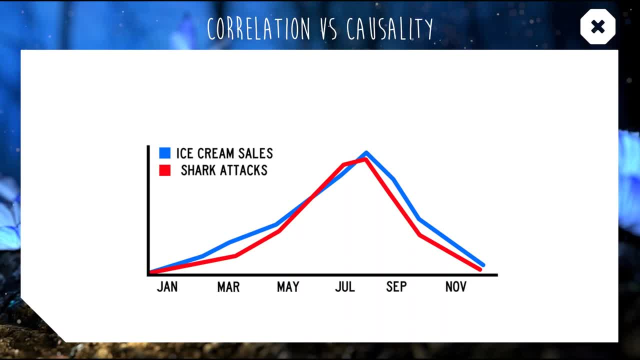 So here is some data that I found on a stats website called Google Images. it shows the records of shark attacks and ice cream sales over the last year. So that's how you do it, piece of cake, as long as you can remember how to get through. 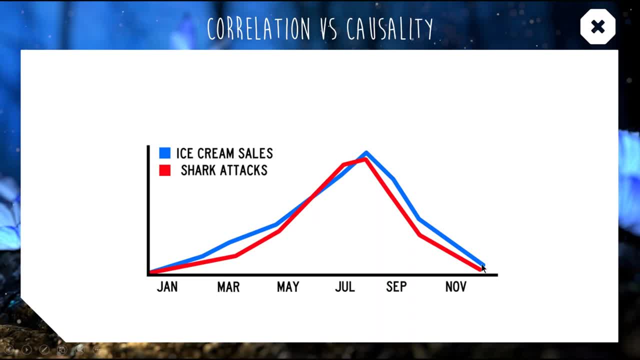 all the options in the menu. So you can see here, over the last year, I've calculated over a 12-month period. Okay, Now what this shocking data is saying, and what Fox News would report, is that ice cream sales are causing shark attacks, or vice versa. 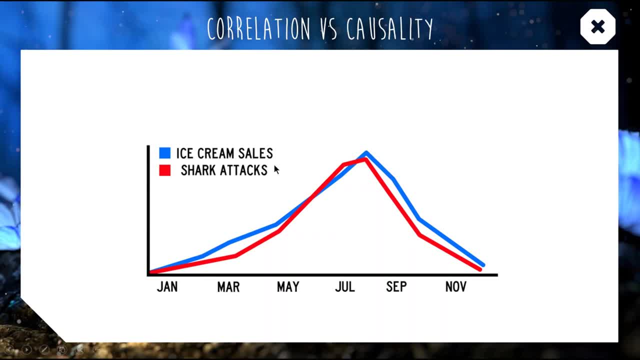 Okay. So what's happening here is that these two variables are mathematically correlated. All right, if I put these two into a calculator from here to here, you would see a correlation of a very, very strong effect. Okay, Just because two variables are correlated does not mean that one is causing the other. 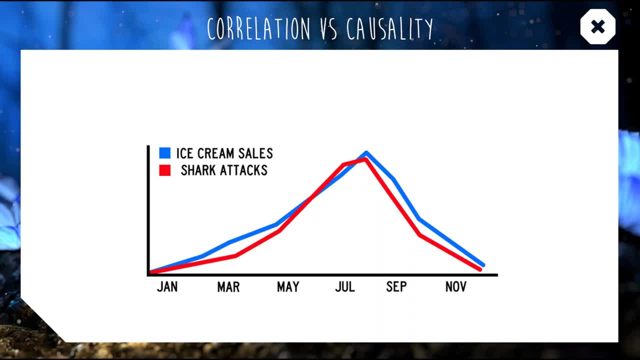 is where you need to ditch the calculator and use a bit of common sense. there's no common sense link between ice cream sales causing shark attacks or vice versa. okay, these two are linked together because they are affected by the weather. okay, in the warmer months, more people are swimming, so 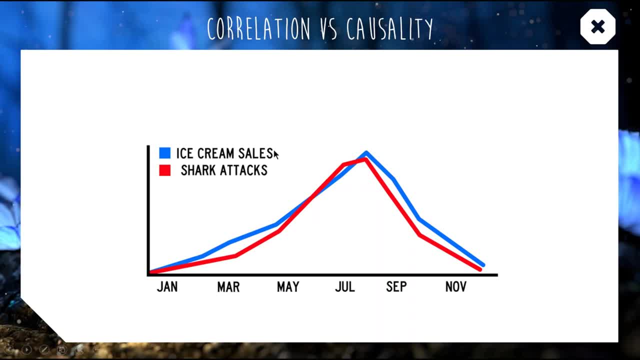 there's more shark attacks and in warmer months more people buy ice cream sales. okay, so sometimes you can have two variables which are correlated because they are caused by similar things, so there's a third party causality, or sometimes you can have one variable causing the other. 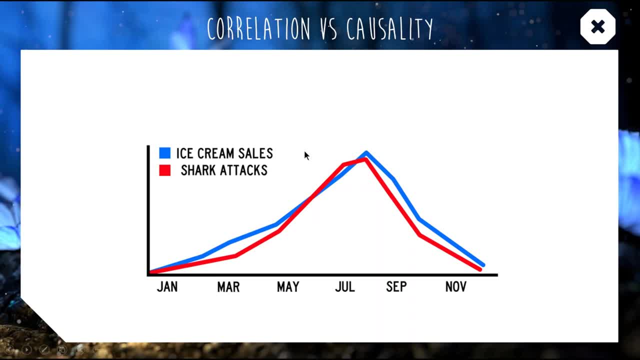 or vice versa. okay, in my data that i showed you before, there was a correlation between my drinking habits and the weather. okay, obviously, this is because in the warmer months, or warm, warmer weather, uh, potentially i might be sweating more, i need to replenish more liquid, so i'm drinking more. okay, so there was a causality one way, but not both ways, okay. 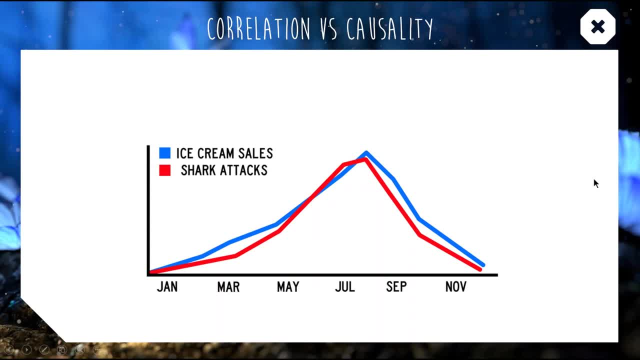 so just be Mindful about responded, just be Mindful about currently. Be mindful that just because data is correlated doesn't mean they're causing each other. There's a really cool website I found that tries to sort of exemplify this. I think it's called Spurious Correlations. 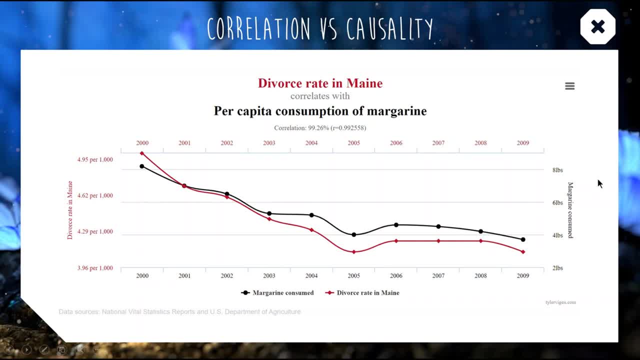 I'll link it in the description below. It'll be just below the like button, just to the left of subscribe, Two buttons which you're hopefully very familiar with. So here we have some data recording divorce rates in Maine, which is an American state. 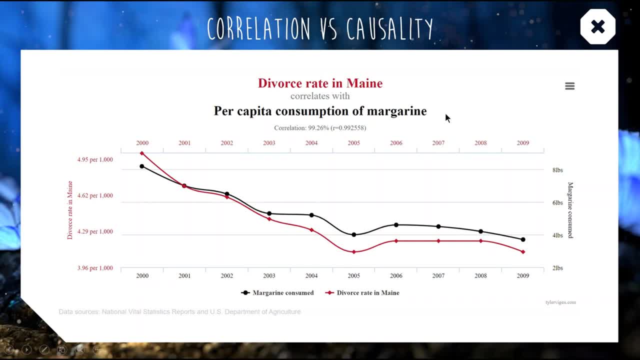 and per capita consumption of margarine. And what's freaky about these two is that you can see here they're very, very similar. They have a correlation value of 0.99, so they're almost perfectly correlated. But there's no logical link between divorce rates and margarine, is there? 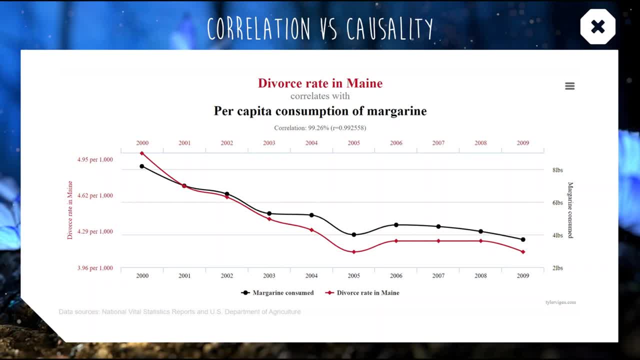 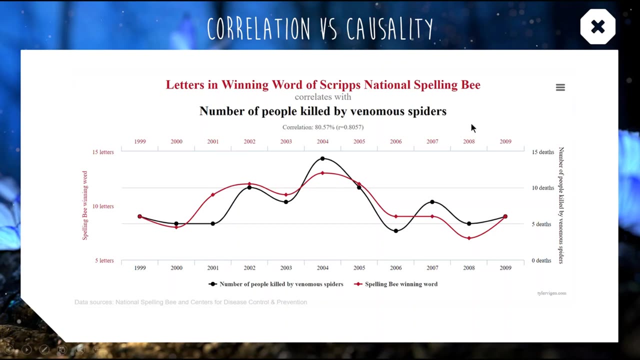 It's just a really, really weird coincidence that these two are almost perfectly correlated, with seemingly no causality whatsoever. Okay, here's another good one. This is the Number of letters in the winning word at a spelling bee correlating with number of people killed by venomous spiders. 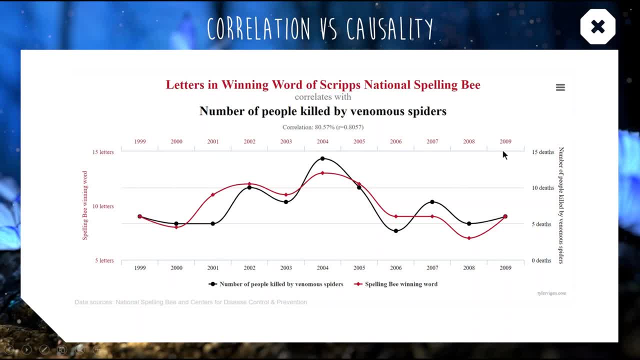 A correlation of 80%. a very similar look in graphs. but if you can find any link between number of words in a word and number of venomous spider bites, I don't think you'll find one. okay, Really close correlation. exactly no causality.